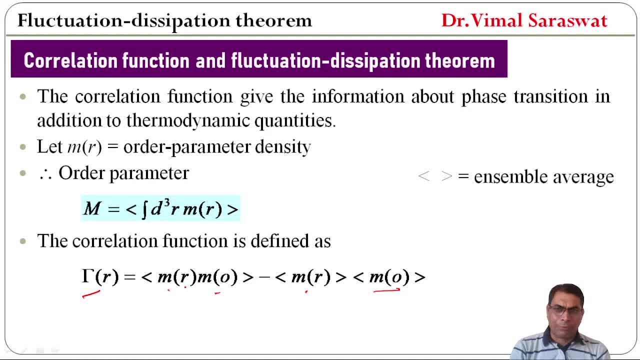 So we have defined the equal English stripped. So correlation function is defined by gamma r equal to ensemble average of m r m naught, minus ensemble average of m r into ensemble average of m naught. So this is actually our correlation function. This function measures the persistence of memory of spatial variation in the order parameter. 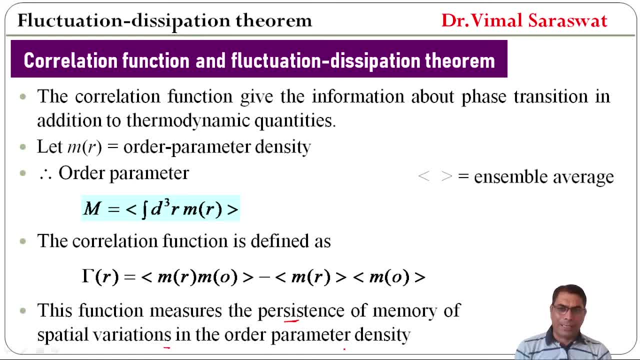 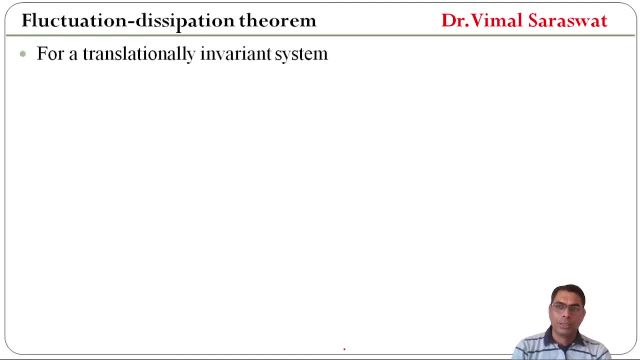 density. So this correlation function measures the persistence of memory of spatial variation in the order parameter density For a translationally invariant system. if our system is translationally invariant, that means we are not getting any kind of change in translation. So this correlation function measures the persistence of memory of spatial variation. 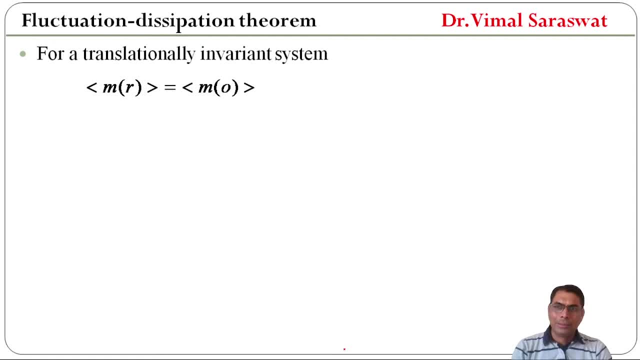 in the order parameter density, then ensemble average of mR is equal to ensemble average of m knot And Gamma-R is equal to ensemble average of mR, m knot minus ensemble average of mR. into ensemble average of m knot, that ensemble average of M R is equal to ensemble average of M naught. 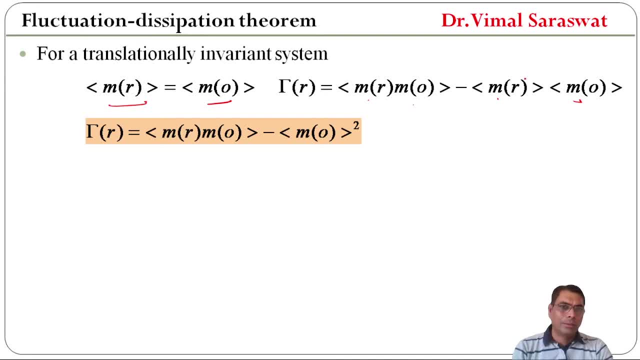 So if we write ensemble average of M naught instead of this, then gamma R is equal to ensemble average of M R M naught minus A square of the ensemble average of M naught. So we will get this correlation function. A Fourier transform is represented by tilde. 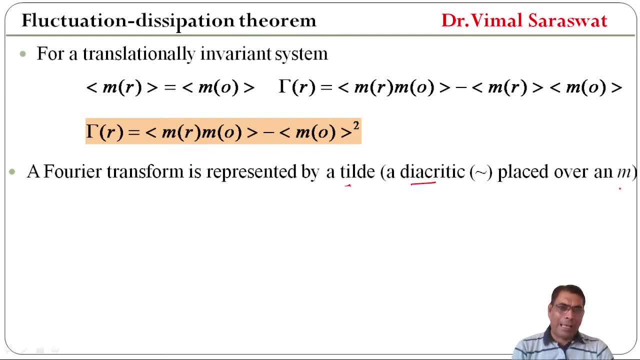 that is a diacritic placed over an M. So if you place a diacritic over this, M means place a tilde. then it will actually be a Fourier transform of M R or M Fourier transform. For example, if M? R is equal to integration: d3k divided by 2 pi, whole cube. 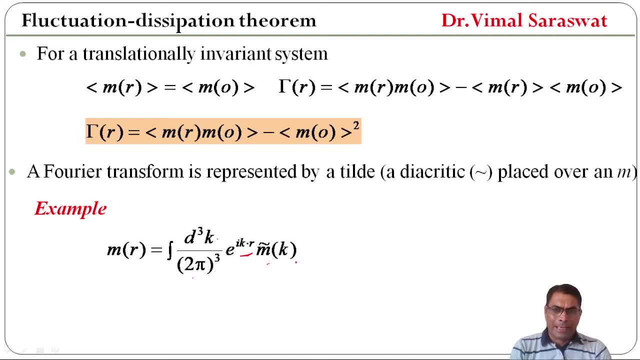 exponential iota, k, dot, R, M tilde k, then if you want to get its Fourier transform, it means you have to get its value. then what will you get? So Fourier transform of M, that is, M tilde k, is equal to. 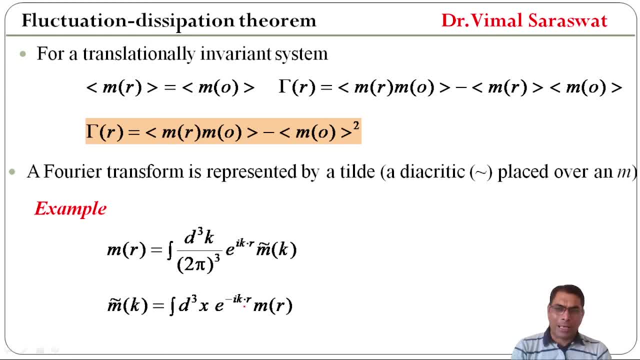 integration: d3x exponential minus k, dot R, M R. so this function, M R, its Fourier transform, will be this: Since M R is real, then M tilde star k is equal to M tilde of minus k, So M R is real. that is why its value will be equal to this. 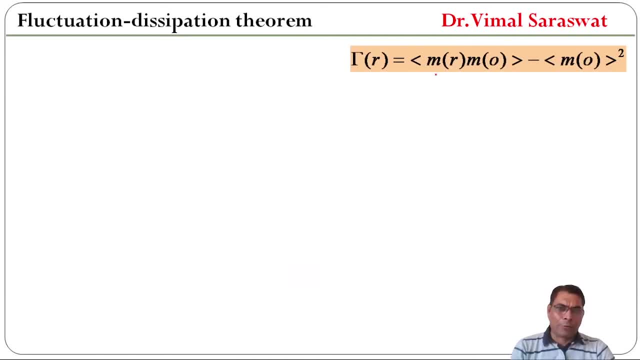 Now, gamma R is equal to ensemble average of M R into M naught, minus a square of ensemble average of M naught by taking Fourier transform on either side of it. Now, if we take Fourier transform on either side of this equation, k. 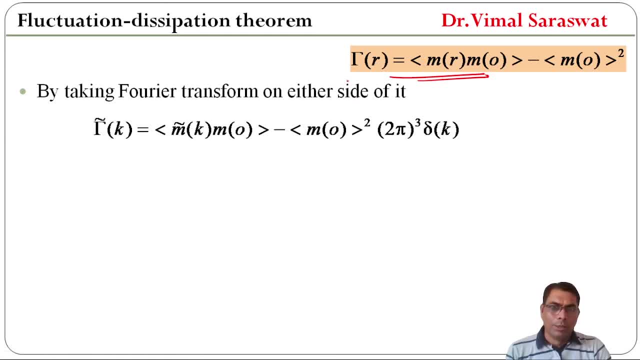 what will you get? So Fourier transform of gamma, that is, gamma tilde k is equal to ensemble average of M R, the average of M tilde k, M naught minus a square of the ensemble average of M naught into twice pi whole cube delta k. 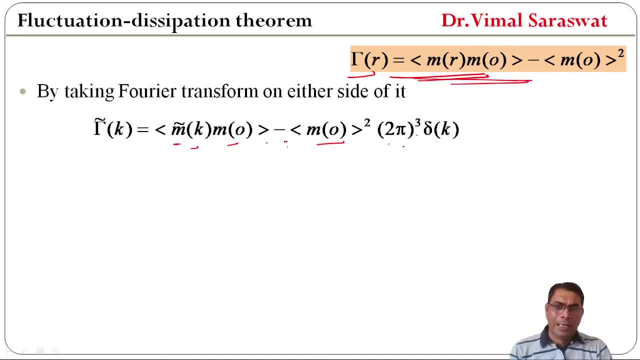 So if we take Fourier transform on either side of this equation k, then we will get this equation, Since ensemble average of M naught is equal to 0, so if this value is 0, then this will be 0,. 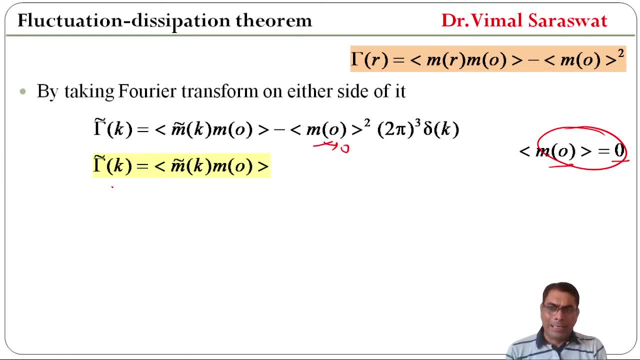 and if this value is 0, then this will be 0,. So gamma tilde k is equal to ensemble average of m tilde k m naught. So we will get this equation: Since m r equal to integration d3k divided by 2 pi, whole cube exponential iota k dot r m tilde k. 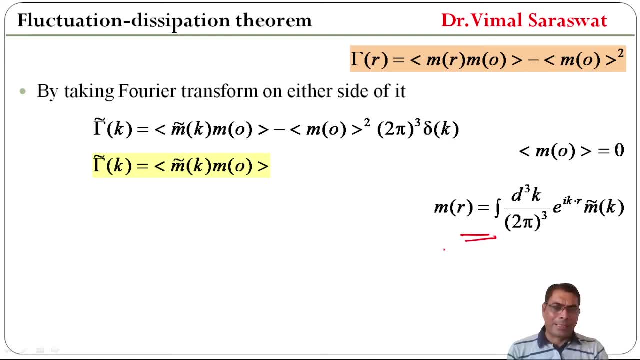 So order parameter density was this. Therefore m naught equal to 2 pi raised to power minus 3 integration d3k. e raised to iota k dot o m tilde k. So we have written o here simply. So m naught is equal to integration d3k and 1 upon 2 pi whole cube. 2 pi raised to minus 3 will be there. 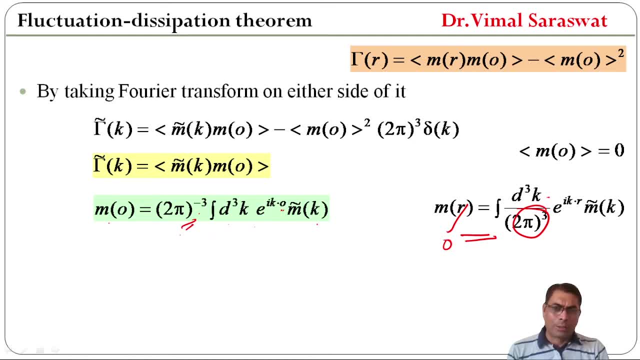 Integration d3k e raised to iota k dot r m tilde k. So m naught equal to integration d3k dot o m tilde k. Also, ensemble average of m tilde k. m tilde p is equal to 2 pi, whole cube delta k plus p. 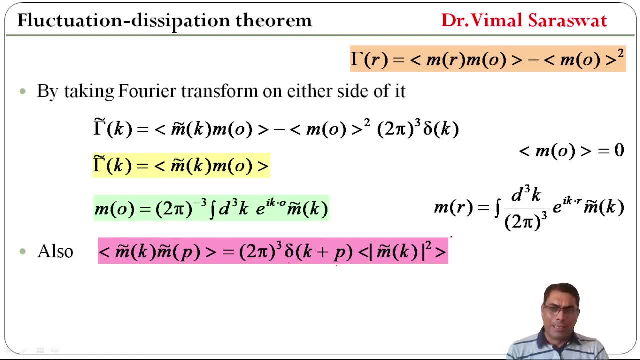 Ensemble average of determinant m tilde k square. Now if we keep values from both these equations here, So by using above equations we get: Gamma tilde k is equal to delta k, magnitude of m tilde k square. So we have written values from both these equations here. 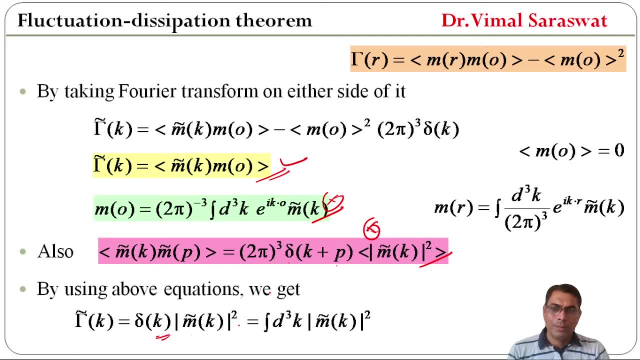 So we have got this And this is equal to integration d3k. magnitude of m tilde k, square And Fourier transform of gamma ie. gamma tilde k is equal to ensemble average of a square of determinant of m tilde k. 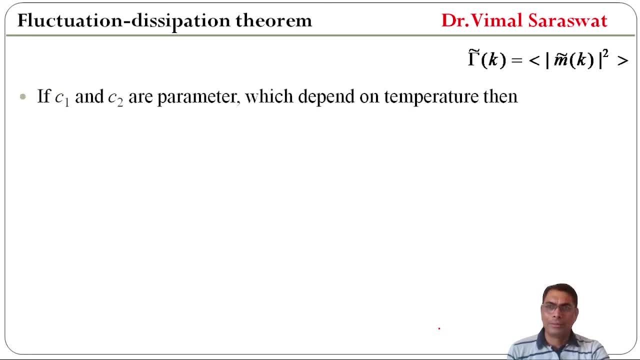 Now we have taken out this equation. If c1 and c2 are parameters which depend on temperature, Now, if c1 and c2 are parameters which depend on temperature, then ensemble average of a square of the magnitude of m tilde k is equal to kt divided by c1 k square plus c2.. 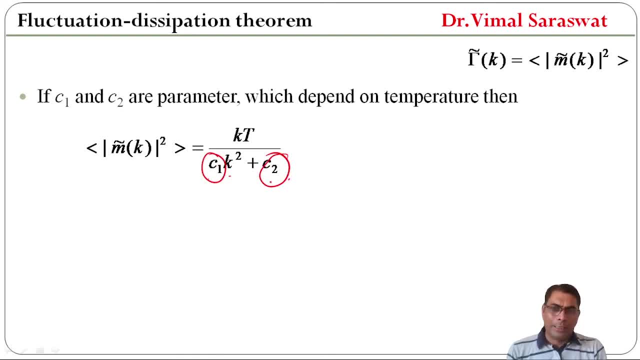 Here, c1 and c2 are the parameters depending only on temperature, and k is Boltzmann's constant, whereas t is absolute temperature. Also, ensemble average of a square of magnitude of m tilde k is actually gamma tilde k. It means this is our gamma tilde k. 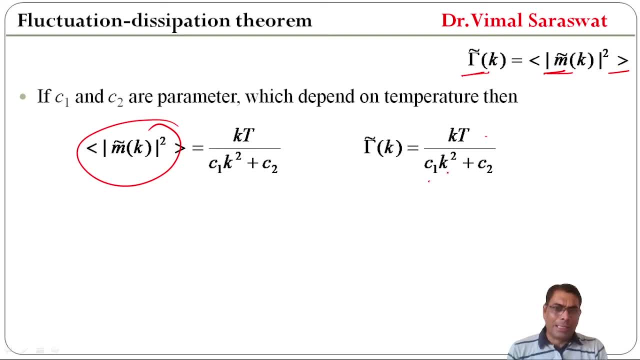 So gamma tilde k is equal to kt divided by c1, k square plus c2.. By taking the inverse Fourier transform we get Now. if we take its inverse Fourier transform, then we will get. gamma r is equal to exponential minus r upon l whole divided by r. 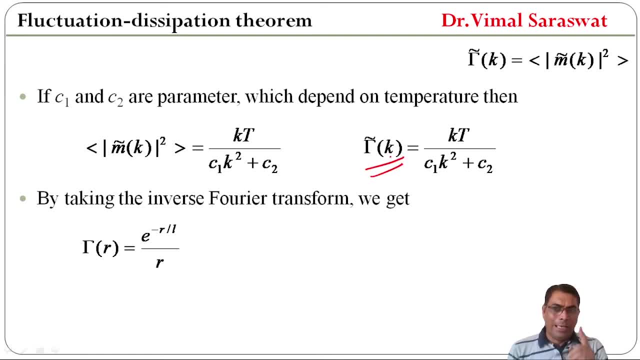 So we have taken the inverse Fourier transform of gamma tilde k. So we have: gamma r is equal to exponential minus r upon l whole divided by r. Here l is equal to a square root of c1.. This is a square root of c1 upon c2 and this is actually correlation length. 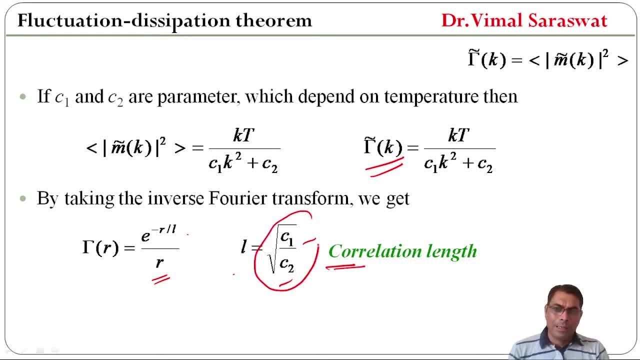 So correlation length equals to a, a square root of c1 upon c2.. The correlation length measures the, a special length. So this is our correlation length, which is used in gamma r, and it is actually measures the a special length. If we take the actor of a square root of r, known as gamma r, this is the length in which the, a square root of r is actually measured. 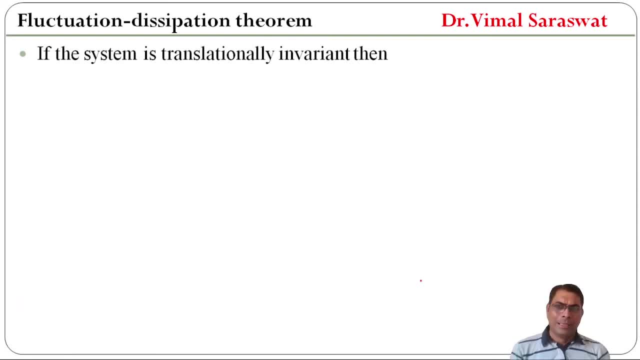 Let's immensitie the coefficient of a quarter root of r squared into c1 over c2.. If the system is translationally invariant, then Now, if our system is translationally invariant, then in that case M is equal to ensemble average of integration D3RMR. 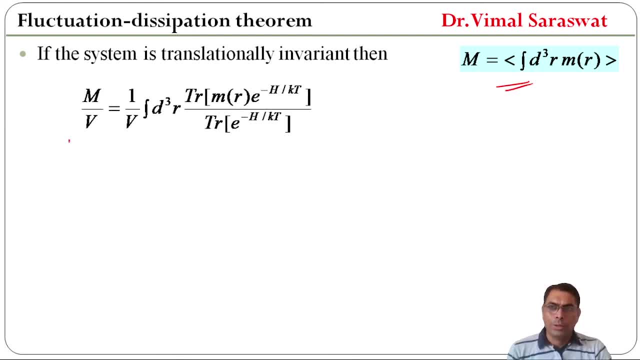 This was taken by M, So M upon V equal to 1 upon V. Integration D3R: trace of MR exponential minus h upon kT Divided by trace of exponential minus h upon kT. So if the system is translationally invariant, then 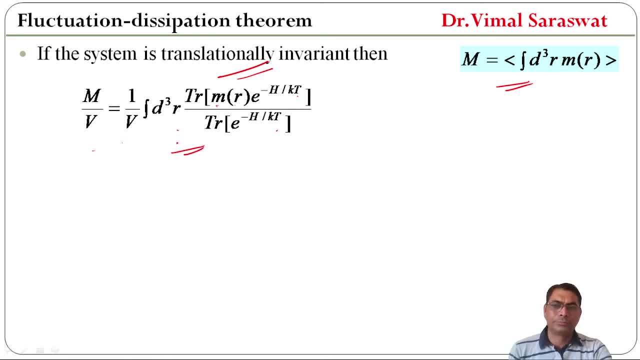 M upon V will be this one, Or this is equal to Trace of M0 exponential minus h upon kT Divided by trace of exponential minus h upon kT, Because integration D3R means V. So this V and this V will be cancelled. 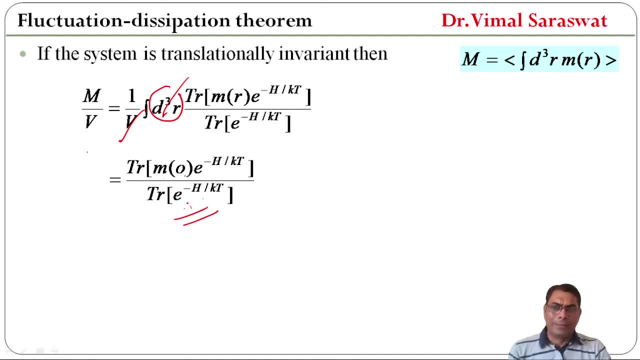 So you will get the value of M upon V. Here h is Hamiltonian, So this h used in M upon V, It is actually our Hamiltonian. If the magnetic field, that is h dash, Is coupled linearly to the order parameter, then 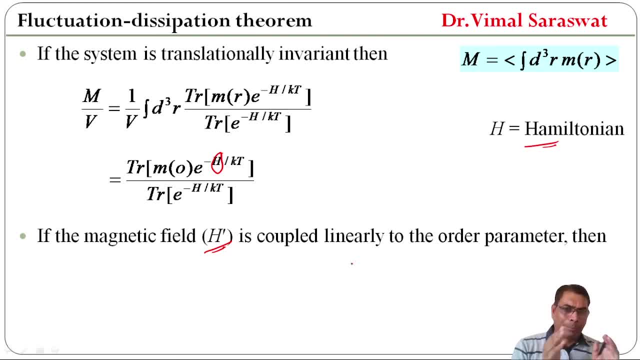 If our magnetic field is Coupled linearly to the order parameter, Then in that case h equal to h0 minus h dash integration D3RMR. And here This h0 is actually Hamiltonian For h dash equal to 0,. 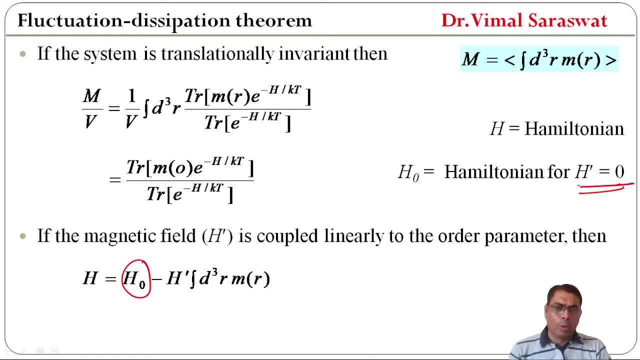 Means when our magnetic field is 0, In that case We have represented the Hamiltonian with h0, So If the magnetic field h dash Is coupled linearly to the order parameter M, Then h equal to h0 minus h dash. integration D3RMR. 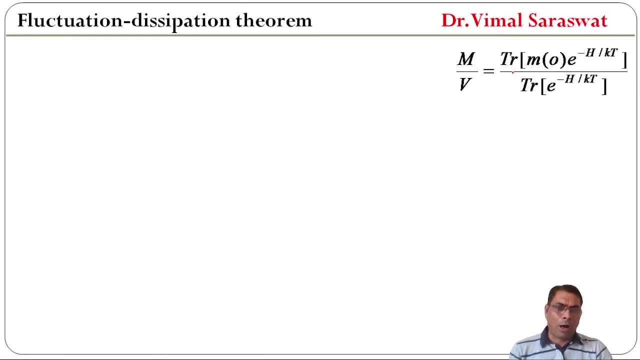 Now M upon V, equal to Trace of M0 exponential minus h upon kT, Divided by trace of exponential minus h upon kT, And HM said That it is Hamiltonian And differentiating this equation With respect to magnetic field, h dash. 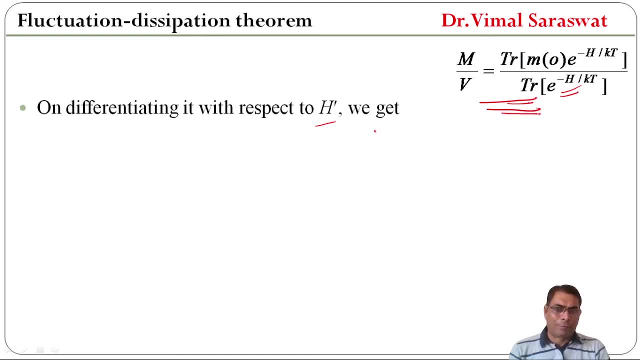 We get Now? If we This equation In respect to magnetic field h dash, We differentiate, What will we get? chi equal to 1 upon kT Integration. D3R Ensemble average of M are M0, Minus. 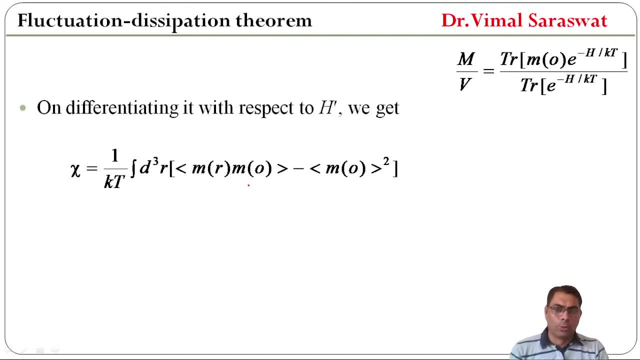 A square of the ensemble average of M0,. So If we differentiate this equation With respect to magnetic field h dash, You will get Chi's value. This, Since Gamma R is equal to Ensemble average of M, are M0,. 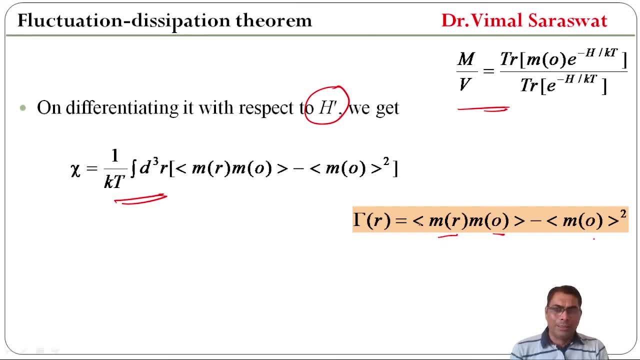 Minus A square of the ensemble average of M0,. This means This is our gamma R. So If we Put gamma R in place of this, Then Chi equal to 1 upon kT Integration D3R. 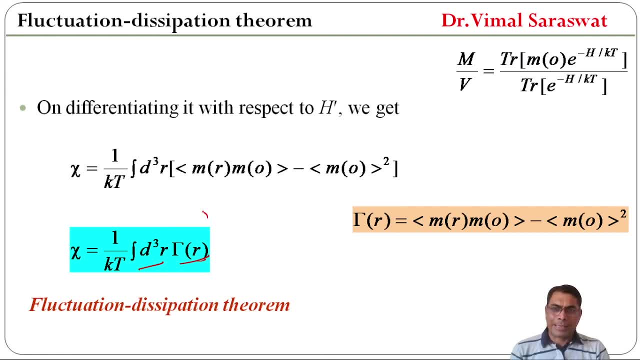 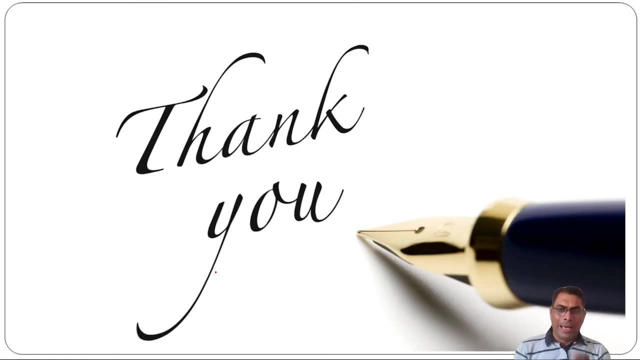 Gamma R, And it is actually Fluctuation-dissipation theorem, And this is our Fluctuation-dissipation theorem And It is a powerful tool In statistical mechanics. So Here we end our session In today's session of statistical mechanics. 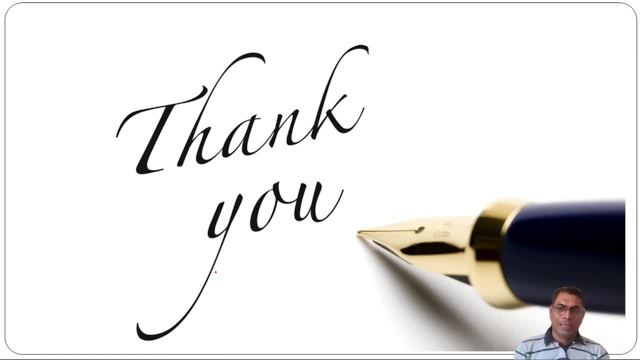 We have discussed about Correlation function And Fluctuation-dissipation theorem, So Good bye.